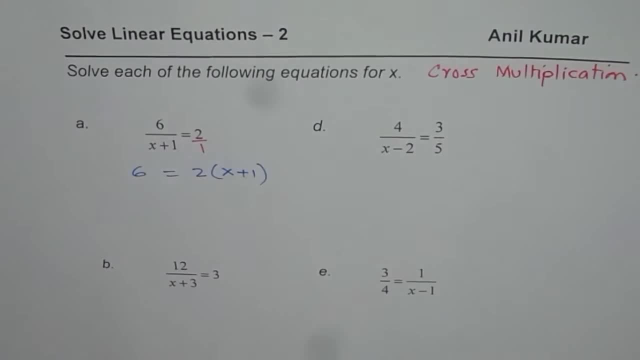 2 times x plus 1.. So that is what cross multiplication is. So now you have a linear equation You can solve, as you have been doing for solving linear equations. After this we will talk about cross multiplication. After this, we have two ways to solve it. Let me show you both. Let me show you both ways to solve this particular equation. So I will rewrite this equation. 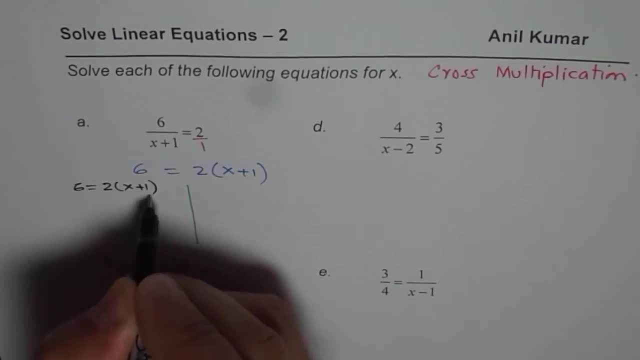 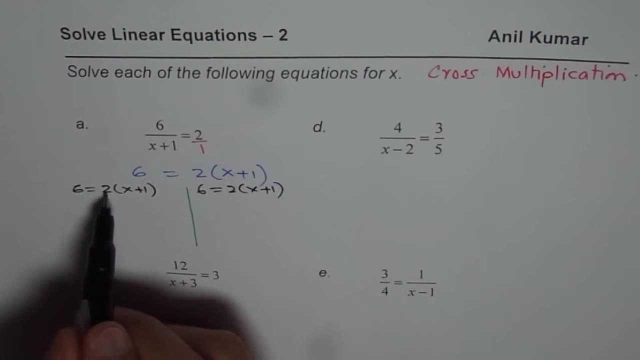 We have 6 equals to 2 times x plus 1.. That is, 6 equals to 2 times x plus 1.. One way is, since you can easily divide 6 by 2 without getting decimals, we will do so. We will divide 6 by 2. we get 3 equals to x plus 1, and then we will take away 1 from x. 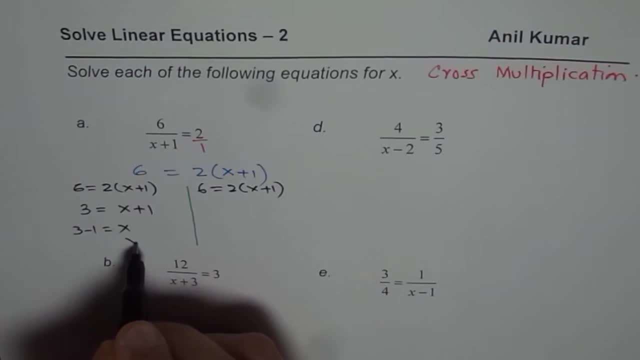 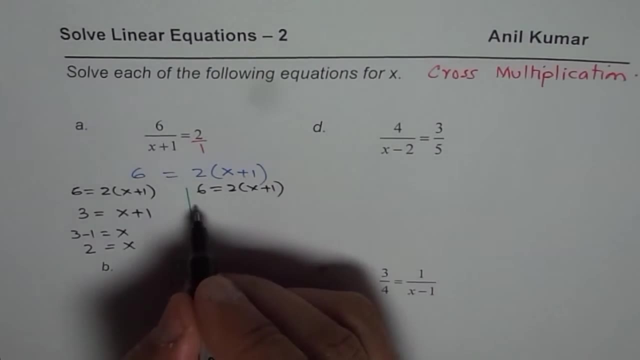 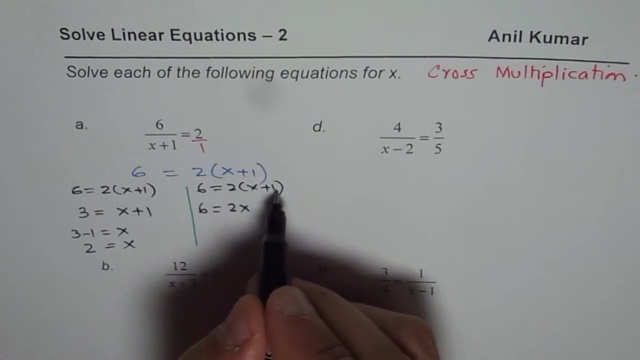 We will take away 1 from both sides, That is 3 minus 1 should be x. So x is equals to 2.. That is one way of solving. The other way is expand the right side, So we have 6 equals to 2x. Distribute a property 2 times x is 2x, 2 times 1 is 2.. So plus 2.. 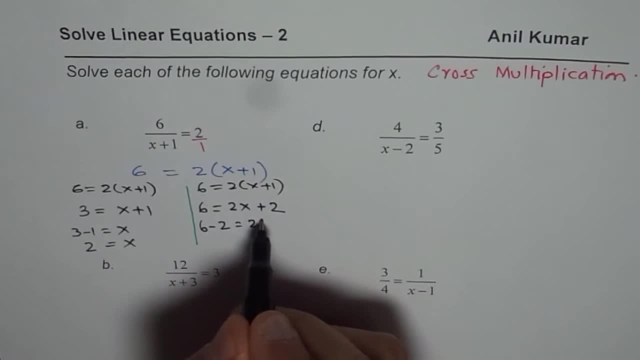 Now take away 2. So we get 6 minus 2 equals to 2x. 6 minus 2 is 4.. 4 equals to 2x. And now divide by 2. So we get x equals to 2.. The same answer, Correct. Exactly the same answer: x equals to 2.. Adopt any method you want, Correct. 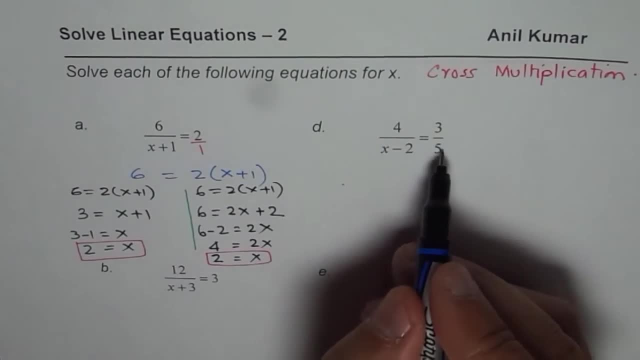 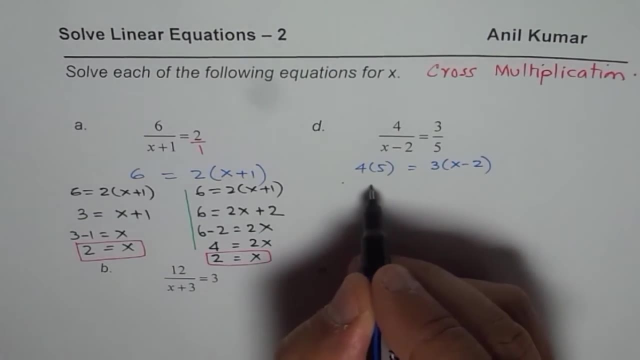 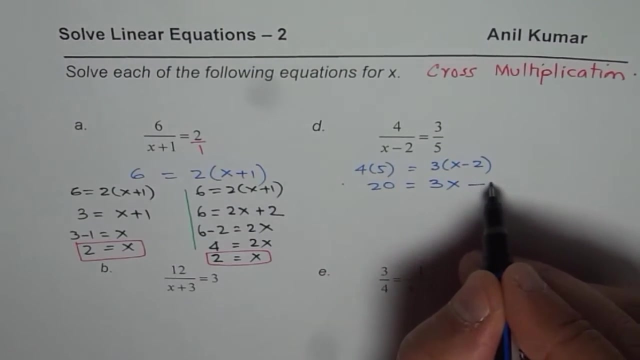 So now let us do this question also. Cross multiply means 4 times 5 equals to 3 times x minus 2.. 4 times 5 is 20 equals to 3 times. Let's open this: 3 times x is 3x minus 6.. 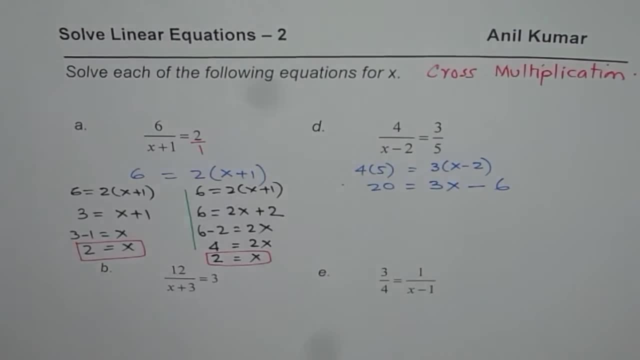 Why did I do that? I did not divide this time, Since I will get you know a decimal which I do not want to work with, Or I am going to get fractions which I am avoiding, Right? So that's the whole idea. So don't divide. in this case, That was good, Since 6 is a multiple of 2.. 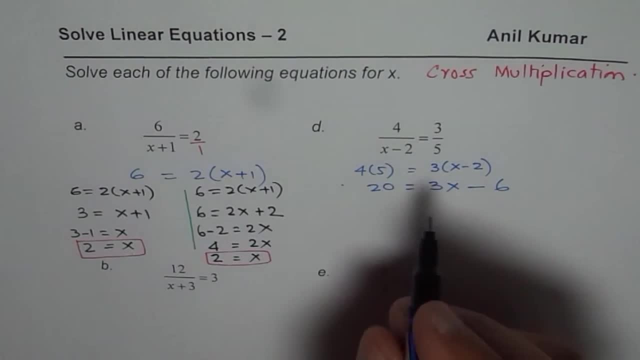 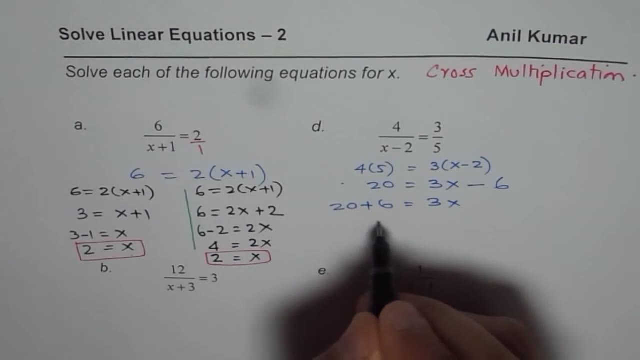 So that was not a bad option right Now. in this case, we will follow the second method, So we will add 6 on both sides, So we get 20 plus 6 equals to 3x, 26 equals to 3x and, of course,